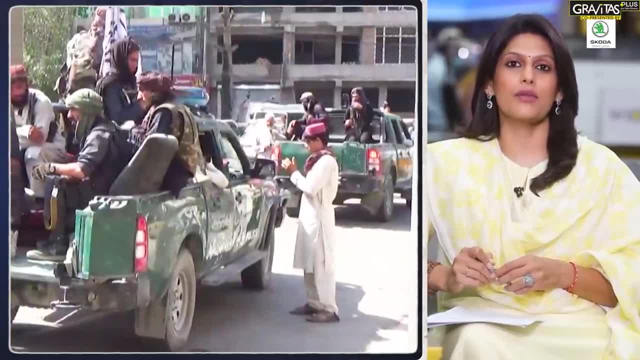 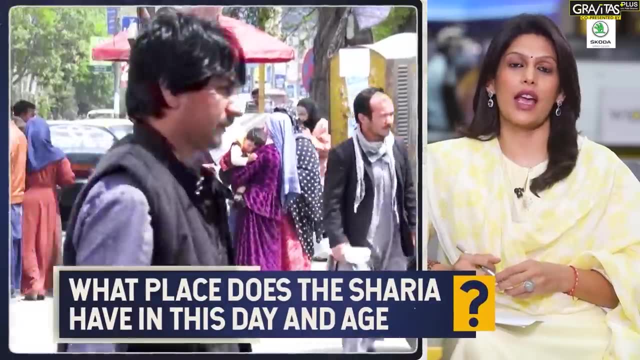 They plan to rule Afghanistan under the Sharia law, under the Taliban's version of the Sharia law. What does that mean? What will change? What will change in Afghanistan? What place does the Sharia have in this day and age? How many people in the world follow it? 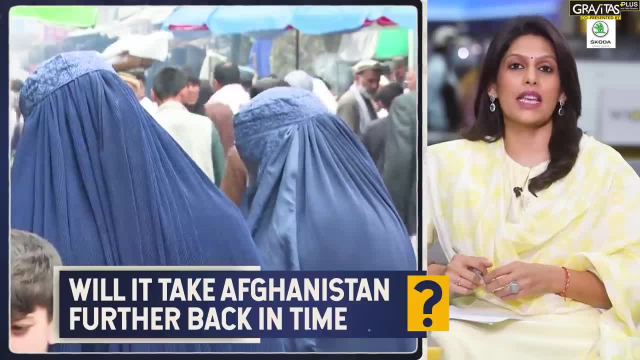 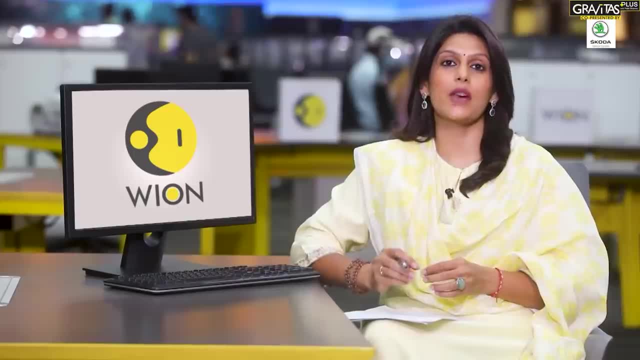 Why is it so controversial? Why does the world fear it will take Afghanistan further back in time? We've spoken to a lot of scholars and experts to put this report together. We'll try to answer all these questions, starting with the first question. 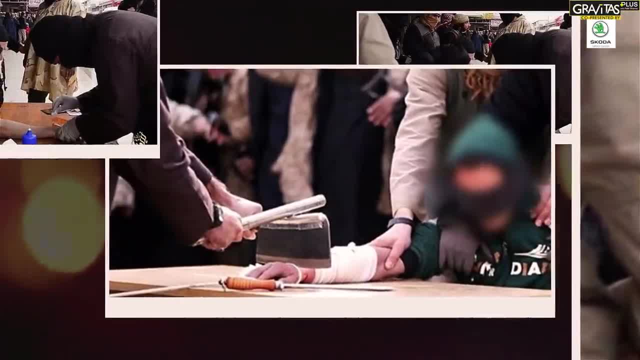 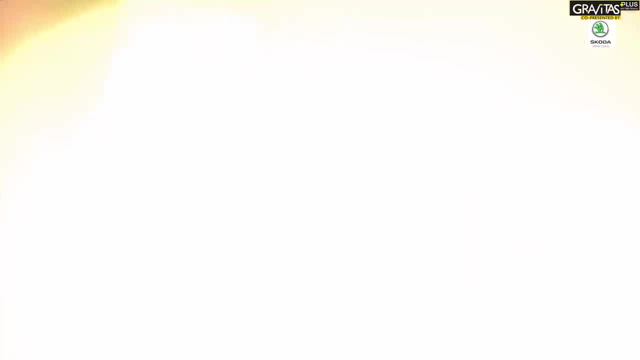 What is the Sharia? To many, the word conjures horrors of hands being cut off, of adulterers being beaten and women being oppressed. In fact, no religious law has ever had worse press as the Sharia has in recent times. Why is that so? 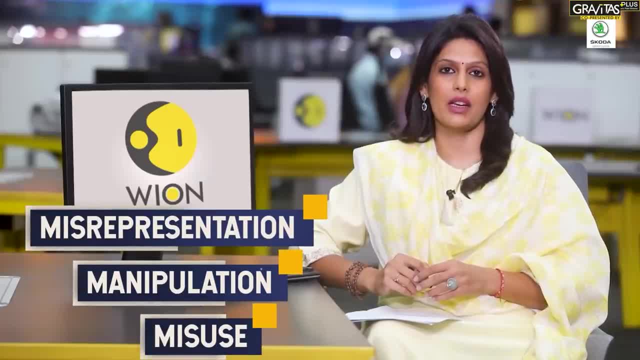 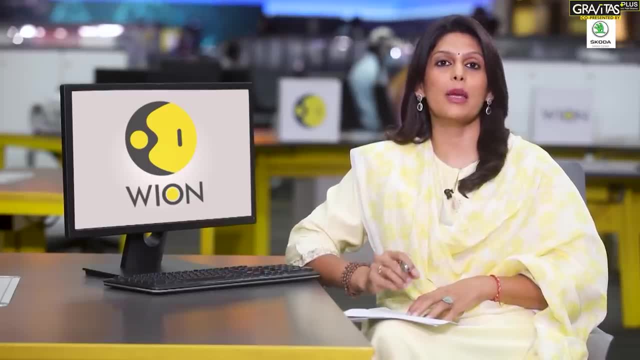 Thanks to the misrepresentation, manipulation and misuse of the Sharia By whom? Islamic regimes, politicians, clerics, radicals, terrorists- They've all used the Sharia to rule in the name of God. So, coming back to the question: what is the Sharia? 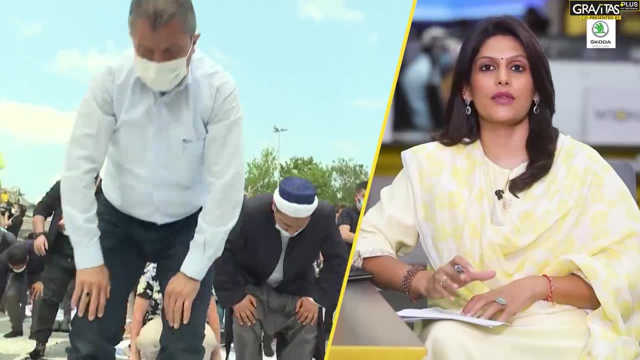 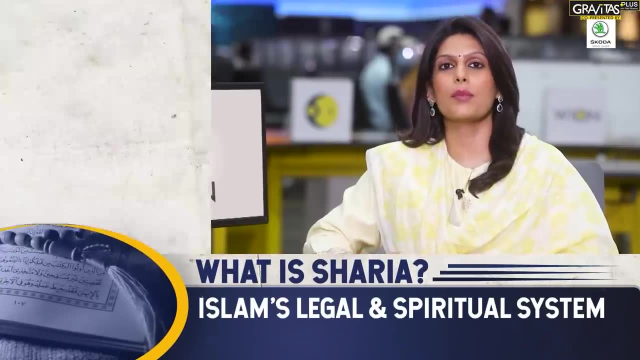 Well, there is no clear definition. Different people understand and apply the Sharia in different ways, But if we put the broad concepts together, this is what a definition would sound like. The Sharia is Islam's legal and spiritual system, both divine and philosophical. 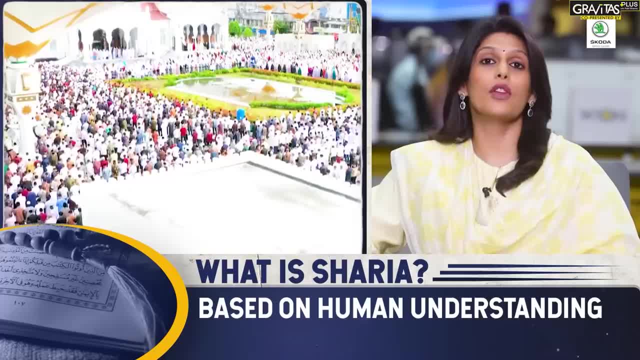 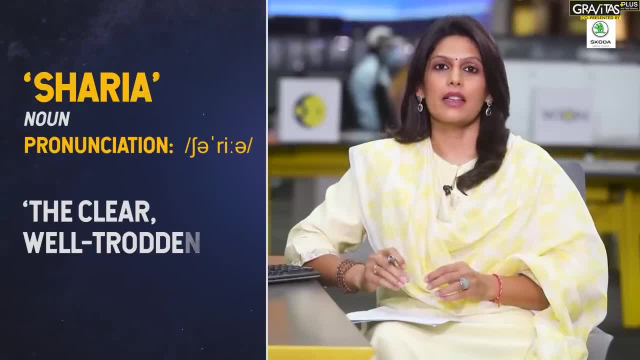 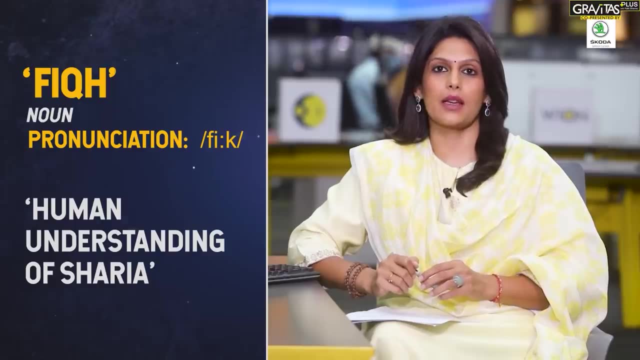 Divine because it is said to be God's will for humankind. Philosophical because it is based on the human understanding of what that divine will is. In Arabic, the Sharia translates to the clear, well-trodden path to water. The human interpretation of Sharia is called the Fiqh. 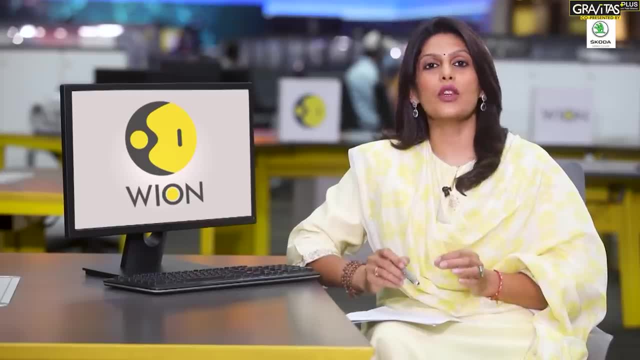 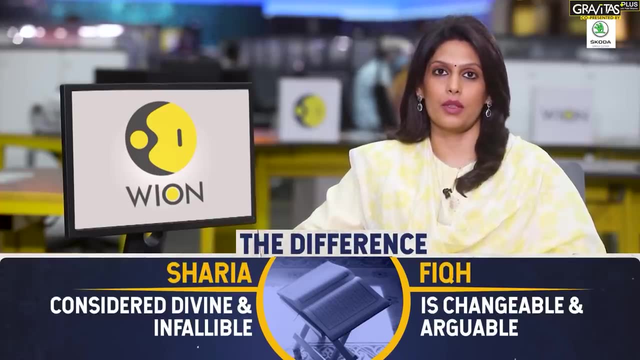 which literally means understanding. Now, these terms are used interchangeably, but they're not the same. Sharia is considered divine, permanent, infallible, But its understanding is human. It's a set of rules put together by Muslim scholars over the centuries. 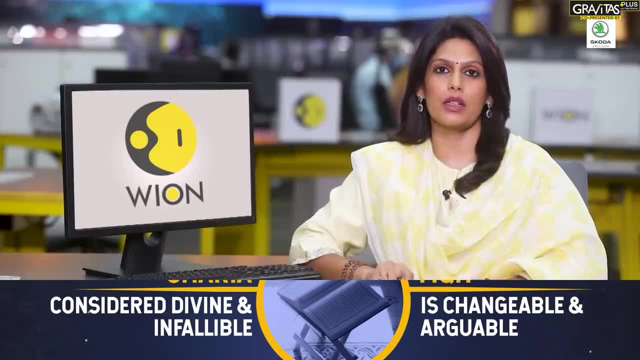 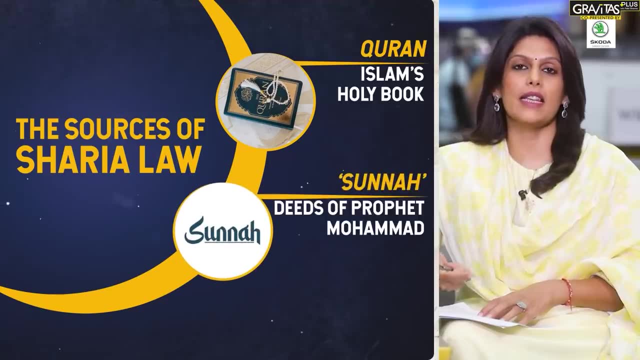 These rules have been drafted and applied to suit those in power. Where do the rules come from? Three sources: the Quran, which is Islam's holy book. the Sunnah, which is basically the deeds of Prophet Muhammad, and the Hadith, the sayings of the Prophet. 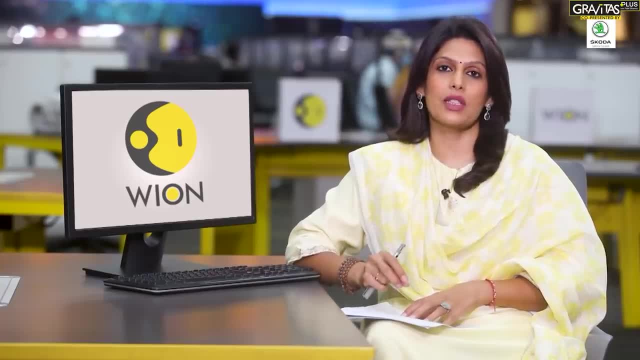 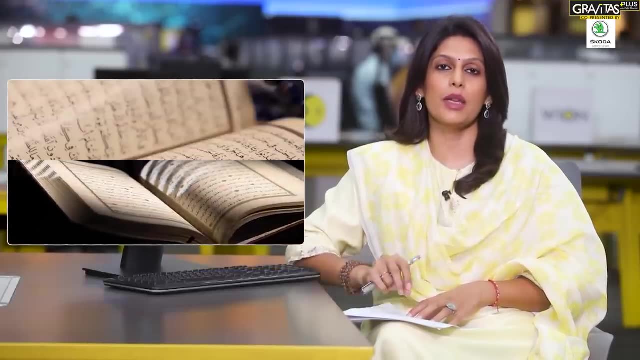 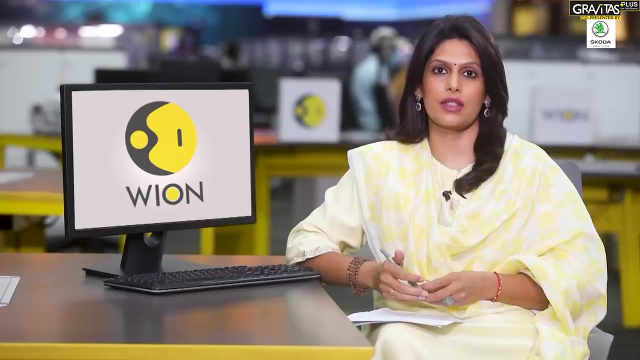 There's a range of other sources to work out how God wants Muslims to live, But there is no single law book, no definite statute, no set judicial precedent to determine what the Sharia is. It's basically a vast collection of different, often conflicting, interpretations. 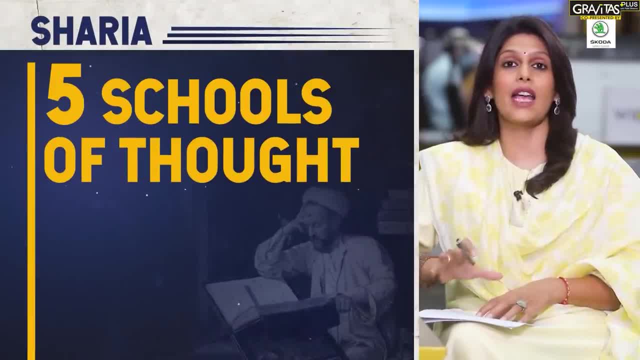 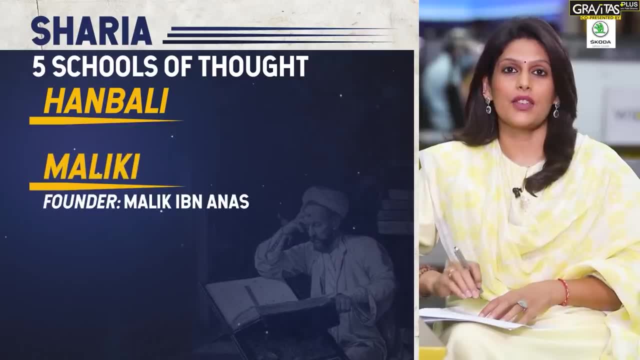 These interpretations gave birth to five schools of thought, five legal schools of Sharia, And you must know this. there are different kinds of Sharia. you would say Hanbali, Maliki, Shafi, Hanafi. These four belong to Sunni Islam. 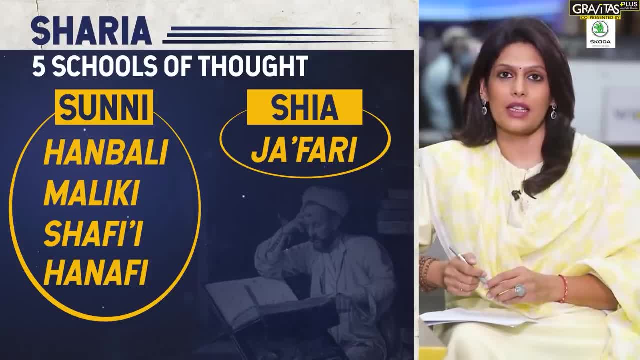 The fifth is a Shia version of Sharia. It's called Jafari. All five of them are named after theologists and jurists- the men who interpreted Islamic texts. Now look at this map. The Hanbali school is the smallest and strictest of them all. 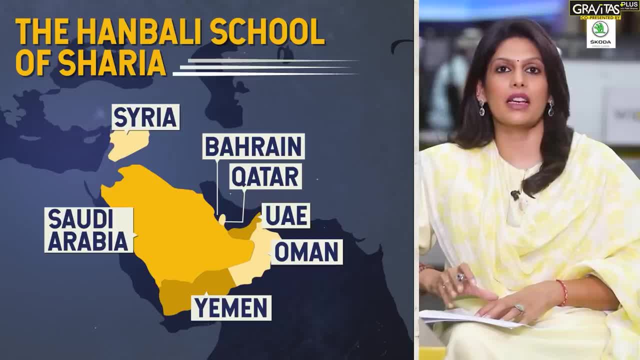 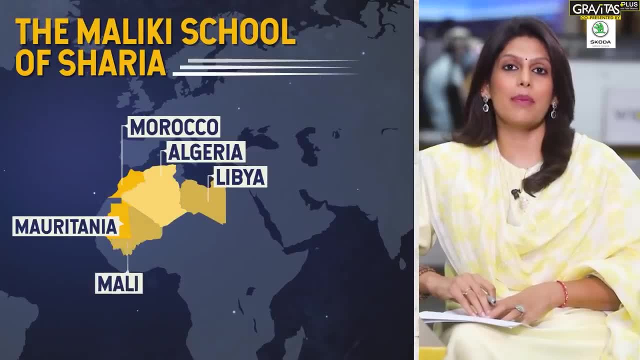 Its primary source is the Quran. It is practiced in Saudi Arabia and Qatar. It also has significant followers in these countries. The Maliki school of Sharia relies mostly on independent understanding of the Quran. It is predominantly found in African nations, the whole of West Africa. 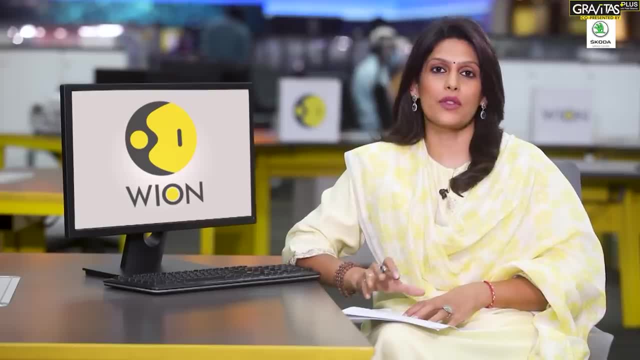 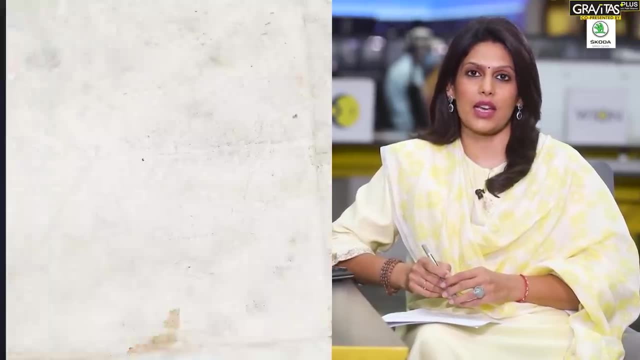 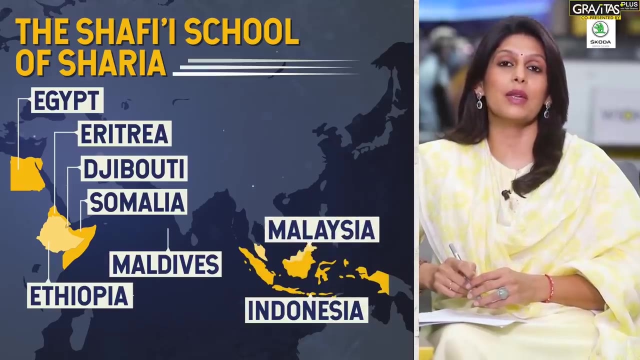 along with Chad, the Sudan and Kuwait. The Shafi school of Sharia relies on consensus over understanding of the Quran, And this is where it's followed East Africa and Southeast Asia, and countries like Somalia, Eritrea, Ethiopia, Lower Egypt, Djibouti, the Maldives, Indonesia and small communities in Malaysia. 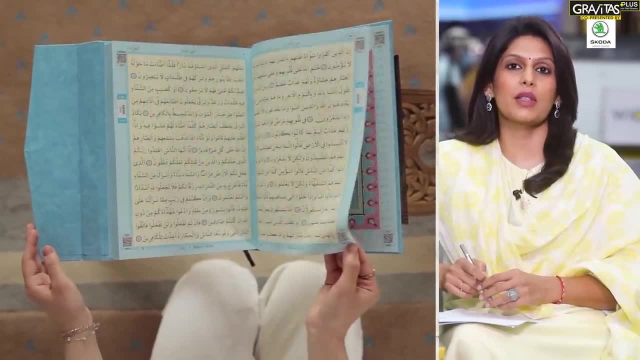 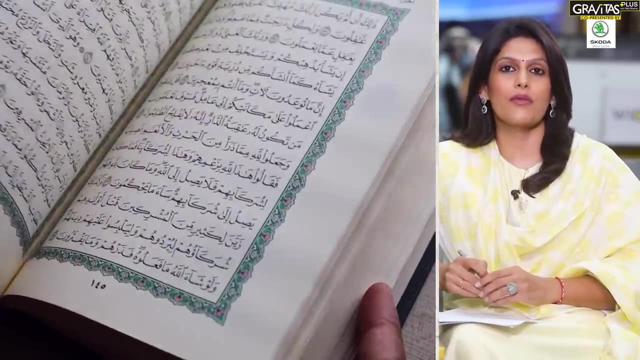 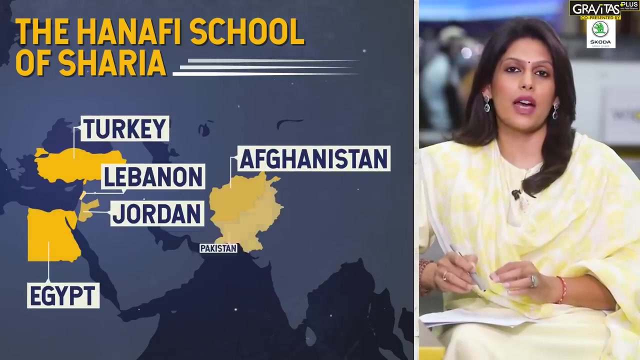 Then we have the Hanafi school, the earliest, the most flexible version of the Sharia. It relies both on consensus and independent reasoning. The Hanafi school has the largest number of followers, approximately one-third of Muslims worldwide. They live in Turkey, Jordan, Lebanon, Egypt, Afghanistan, Pakistan, India and Bangladesh. 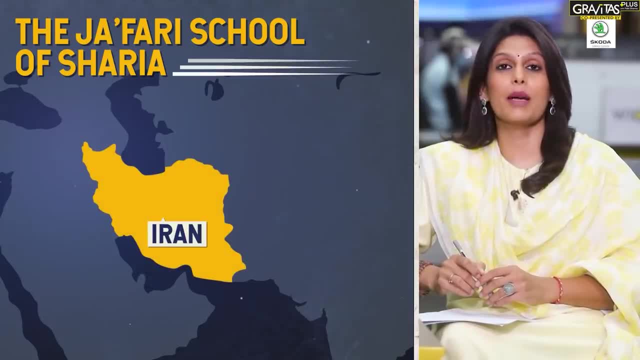 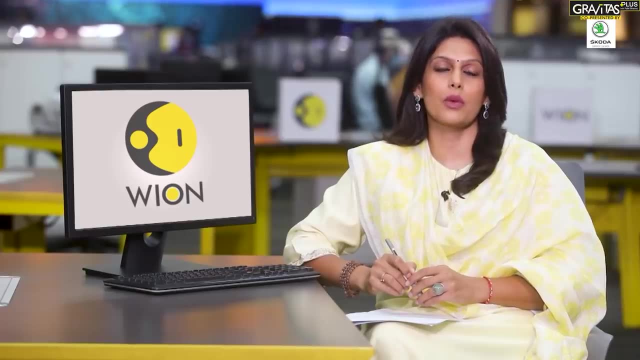 And then we have the Jafri school of thought, followed only by Shia Muslims. It is enshrined in the constitution of Iran. It also has a lot of followers in Iraq and small pockets of followers the world over. So we have five different versions of the Sharia. 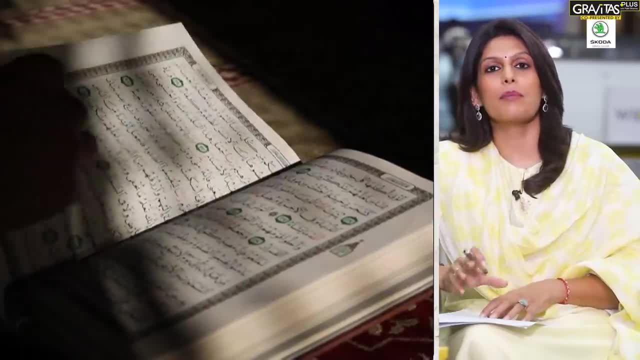 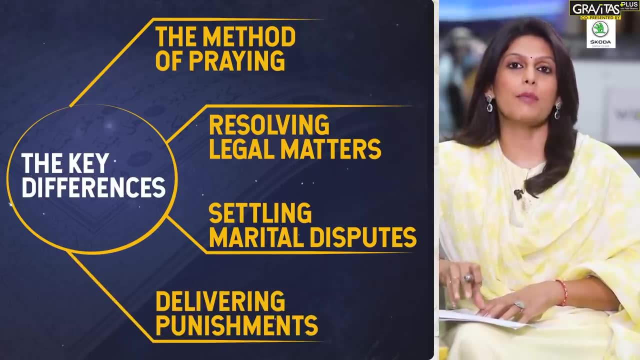 How are they different? Not in the fundamentals of faith, but in their practice. There are differences in how they pray, how they resolve legal matters, how they settle marital disputes, how they deliver punishment for certain crimes, And this is understandable, because no religion is uniform. 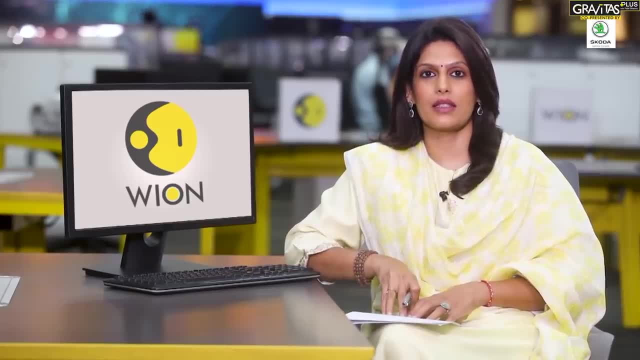 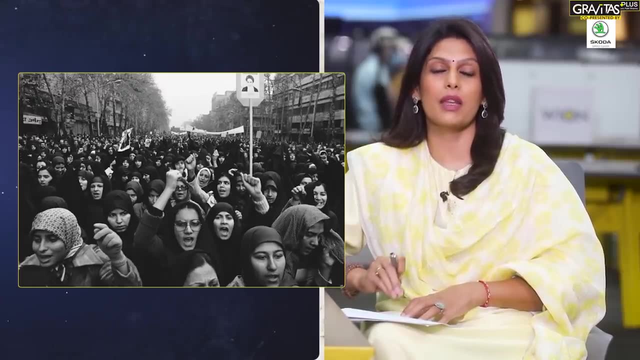 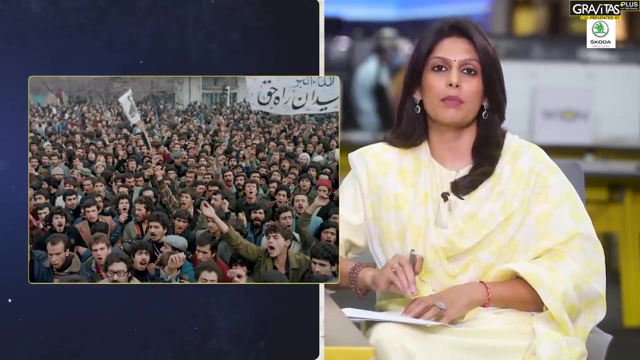 But the problem begins when religion is mixed with governance. Many Muslims who embrace the Sharia thought of it as a substitute for the law of the land, And that's where the problem lies. The Sharia was just supposed to be a way of living. It was not meant to be associated with political power. 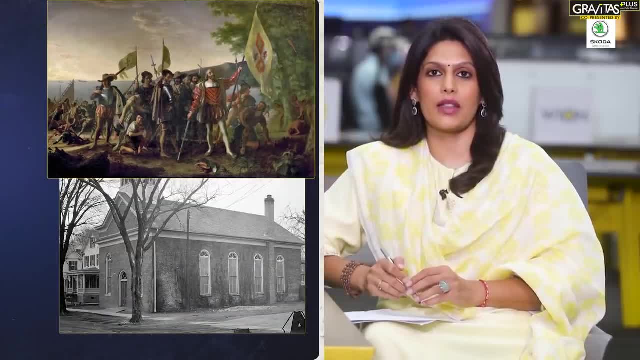 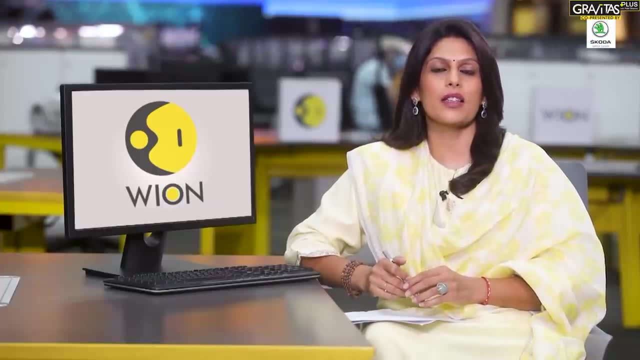 When European colonialism began to spread the crown and the church came together, The church was used to further the interest of the rulers. The same thing happened in Muslim kingdoms, And while European nations later separated the church from the state, many Islamic countries did not. 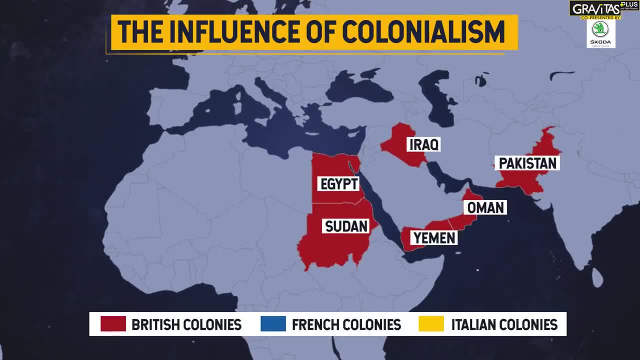 France, Britain and other European powers had colonized much of West Asia, Africa and Asia. When they left, leaders of the newly formed Muslim majority countries faced a dilemma: Should they govern based on previous Islamic values or should they embrace laws inherited from colonial rule? Well, they chose the Sharia as the basis of their legal justice system, And this gave birth to all kinds of theocracies, hardline and moderate Countries like Algeria, Libya, Egypt, the Sudan, Syria, Iraq, Oman, Yemen, Pakistan. they all had the Sharia. 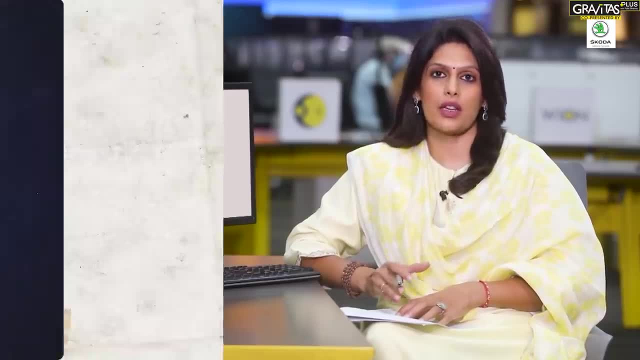 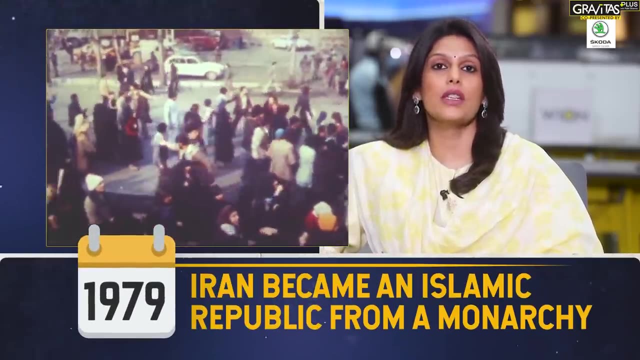 Even countries which were not colonized by the West adopted the Sharia. In 1932,, Saudi Arabia was formed as a theocratic monarchy. In 1979,, Iran witnessed an Islamic revolution. Until then, Iran was a secular monarchy. After the revolution, the clerics took power. 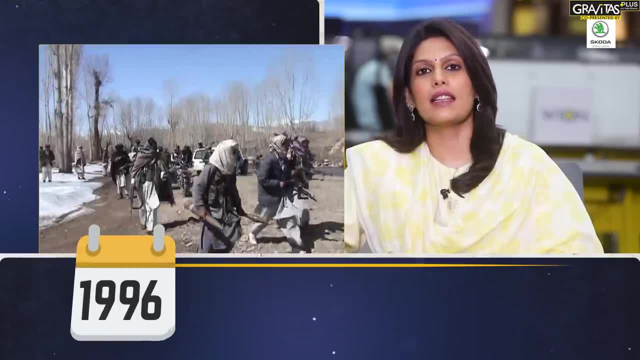 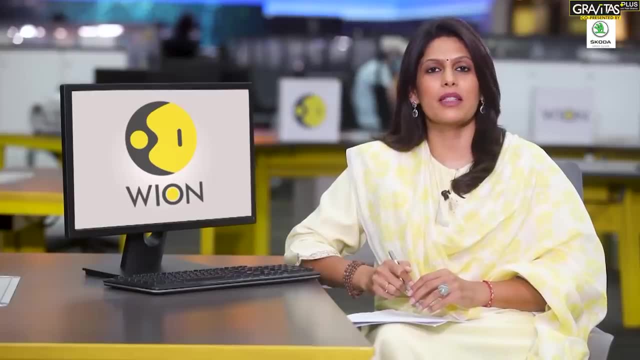 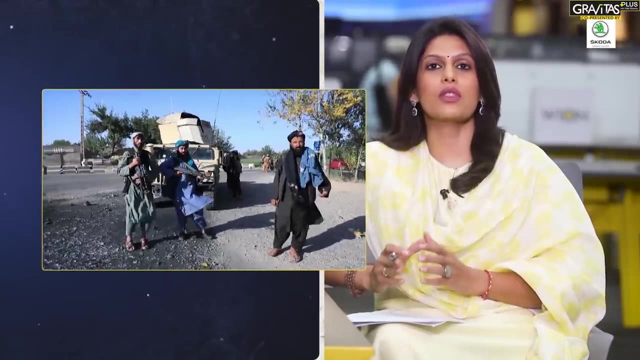 The country became an Islamic republic. Then, in 1996, the Taliban seized power in Afghanistan. They made it a terror regime based on the Sharia. What makes this law acceptable in some countries and horrific in others? Its understanding and implementation. Some countries enforce the most discriminatory and patriarchal aspects of the Sharia. They selectively picked certain verses from the Quran and legalized draconian practices like polygamy, triple talaq, genital mutation. They also enforced rules that had little or no basis in Islam. Research shows that most of these punishments were not sanctioned in the Quran. 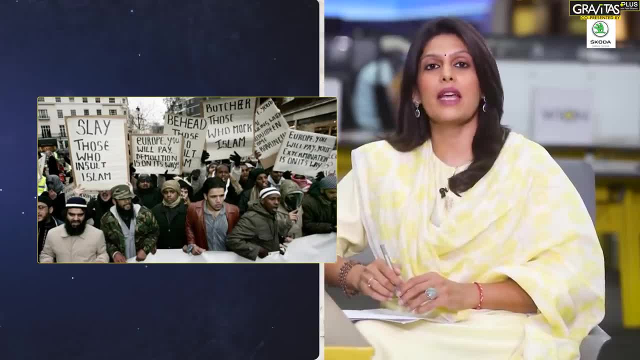 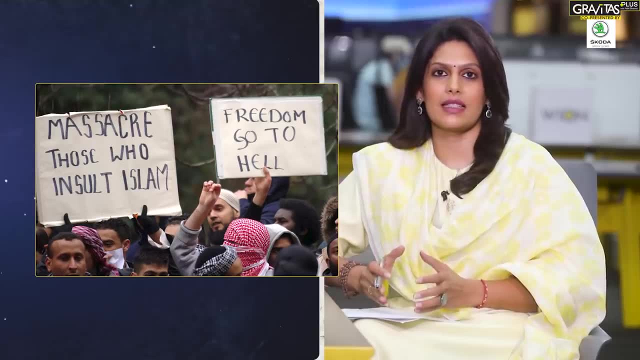 They were not practiced by the Prophet. Yet today they've been made the highlights of the Sharia. They're being used to dictate daily lives of Muslims the world over. A lot of the followers do not understand this. They just stubbornly uphold ignorant and unjust practices. 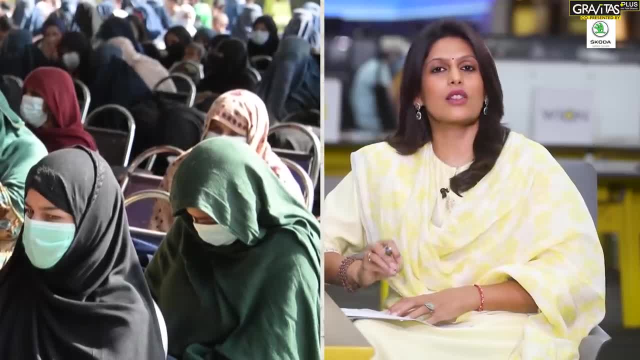 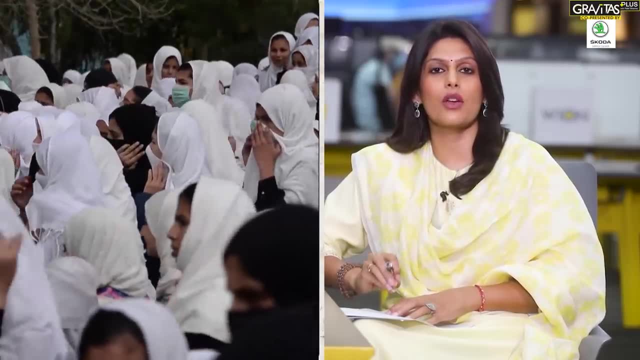 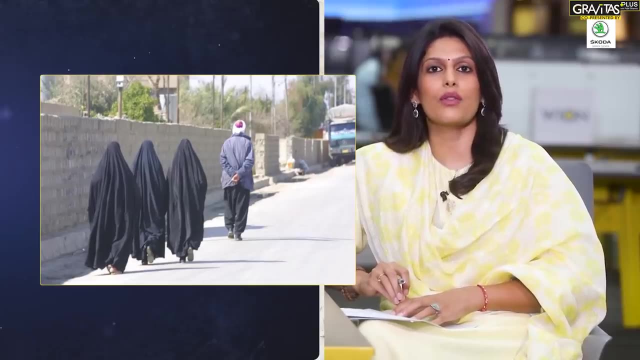 The biggest victims of this are Muslim women. Does God judge differently based on gender? For many clerics it does, Despite the fact that women worked and fought alongside the Prophet. They won't tell you this. In some countries, women cannot step out without an abaya or a veil.